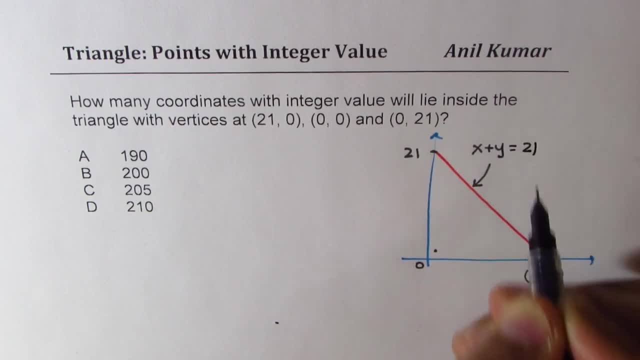 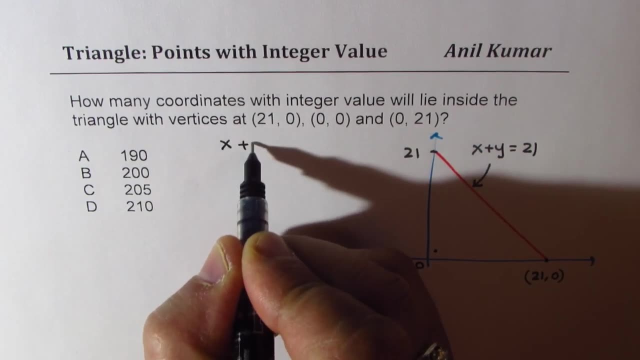 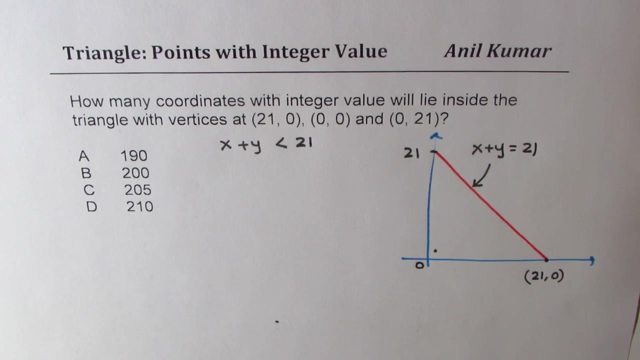 So you could write this as: x plus y equals to 21. So this sum of coordinates is 21. We're looking for points where x plus y is less than 21.. That is what we're looking for, So, and that to incoordinate one, incoordinate one, right. So all positive. So what we notice here is that we can kind of make a series and see the pattern. 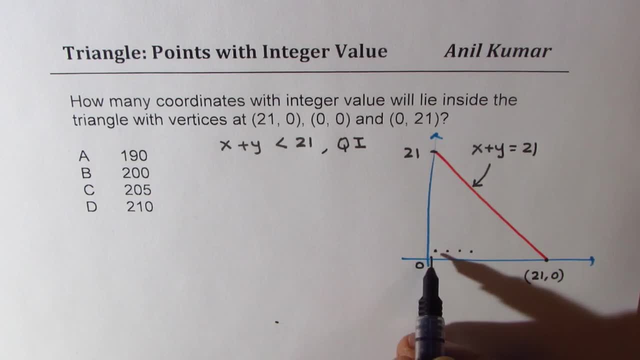 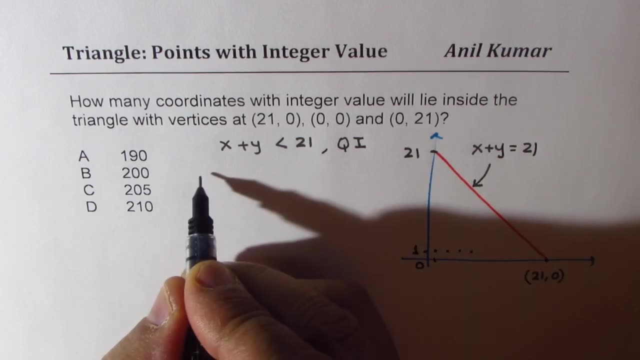 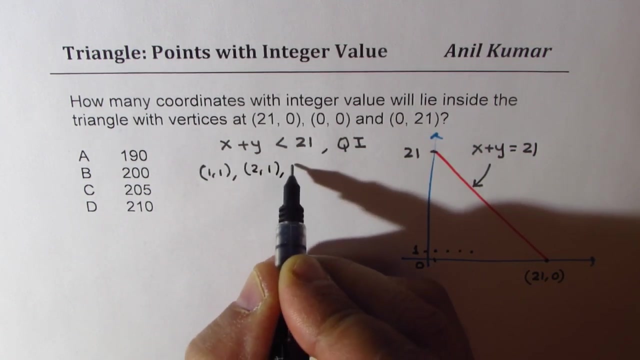 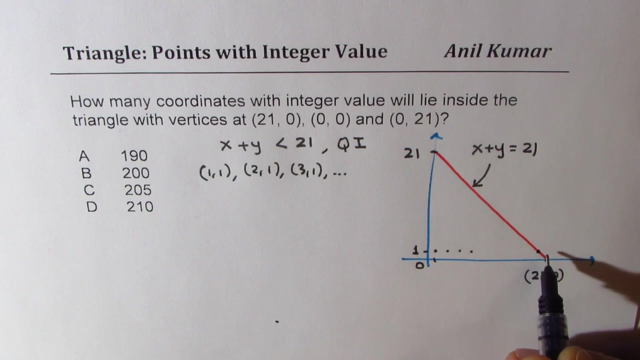 So if I get to the first row where y value is one, let's say this value, y is one. In that case I could get points like: let me write down So we could get one one, y value being one. So two, one, three, one, up to what? So this point here, on this line, will be 20 and one, since the sum is 21.. 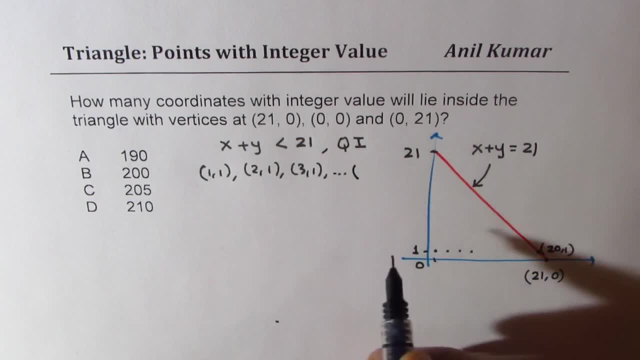 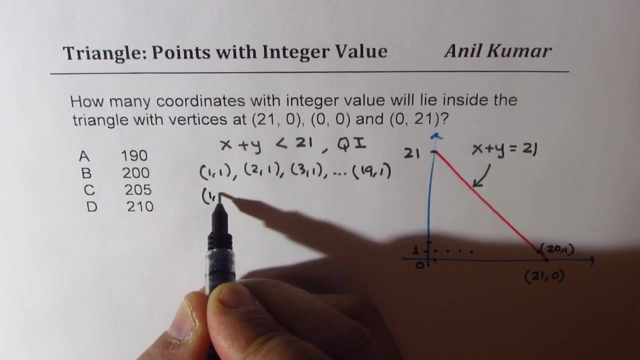 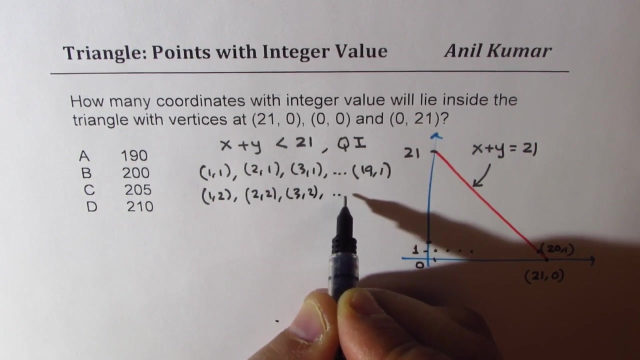 Right, So I'll point before: this will be 19.. One, Do you see that? So we have 19 such points in first row. The second row, let's go to two now- will be y, value being two. So again one, two, two, two, three, two, so on. So this time 18, two will be the last one. 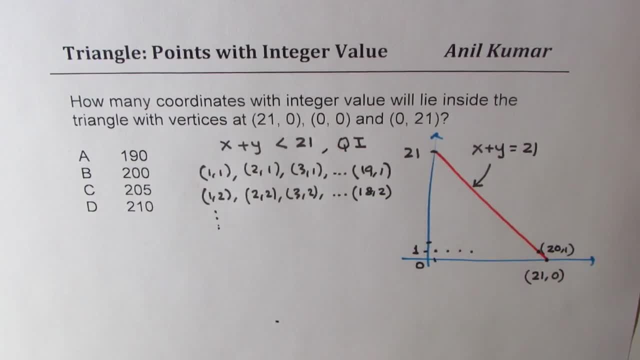 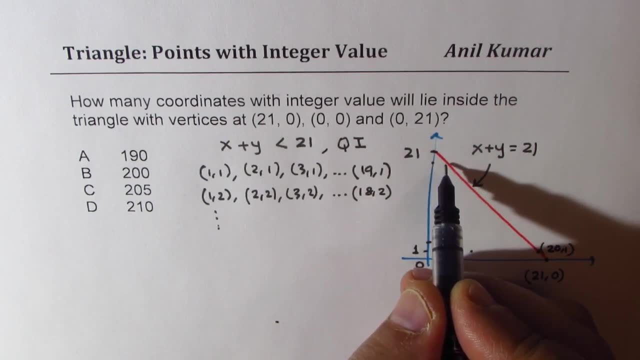 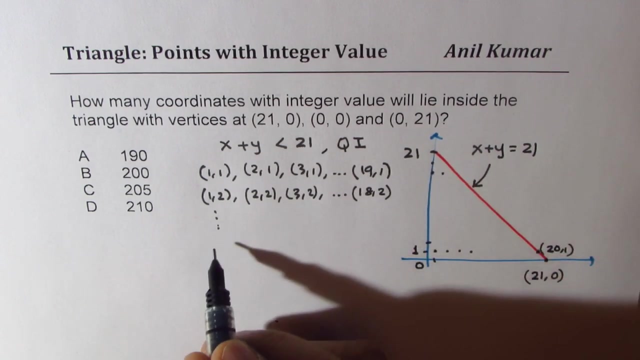 The last point. Likewise you can extend Right. So at the end here we'll have 20, and one cannot be taken Right, But with one we could get 19.. So with with x value of one, we could have 19 as the last point. 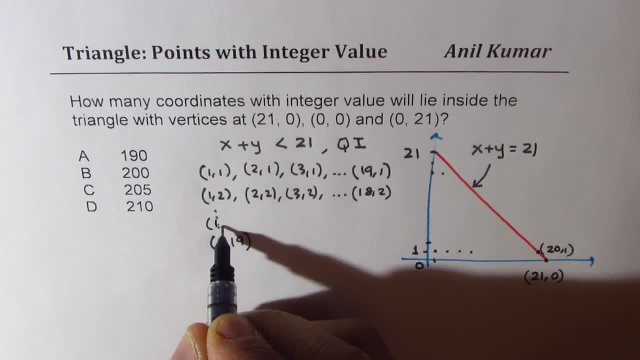 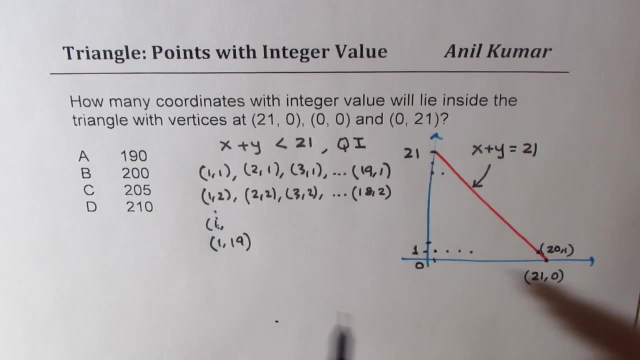 Before this we could have had With one y value of 18 could have done Right. So so what I'm trying to say here is that you could count the number of points. So you will see we'll get two points in this row, Correct. 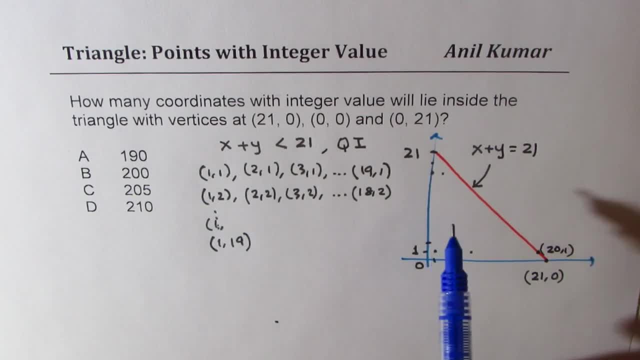 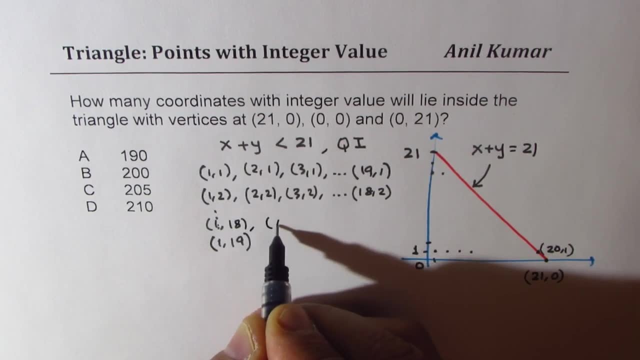 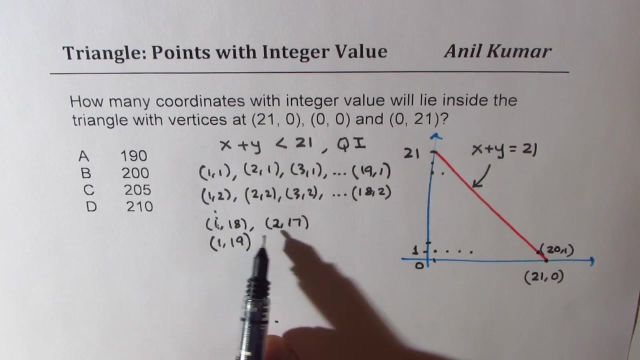 So so the y value will be 18.. Let me write down, Complete this at least. Right. 18 and one With two, It will be 17.. Right, So so that gives you possibly two points Within this particular circle, Right. 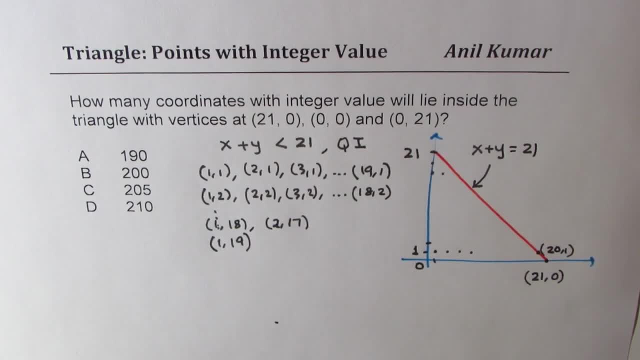 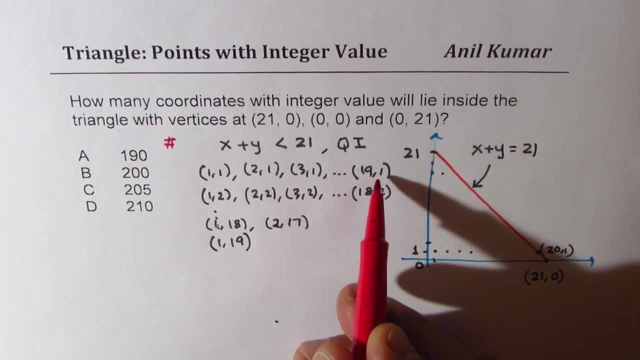 So you have a series here. In the series you will find that the points- number of points- will be How many. let's add them. So one row gives us 19, and then we get 18, and then we get 17, and so on. 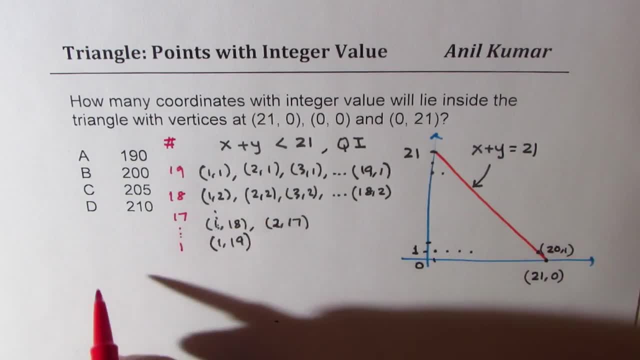 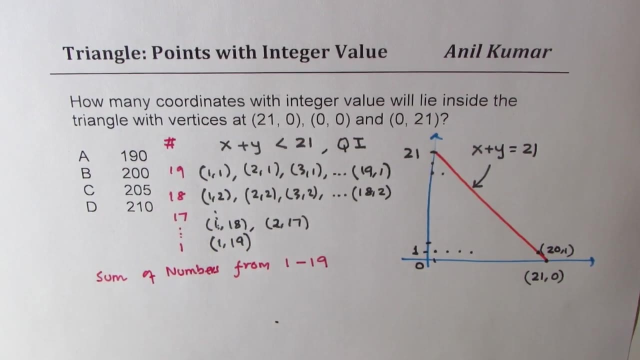 1 till 1. so basically it is sum of numbers, natural numbers from 1 to 19, correct and that you know. you can use the formula here, which is n times n plus 1 divided by 2. now in this case n equals to 19, so what we get here is 19 times 20 divided by 2, which is 190. that 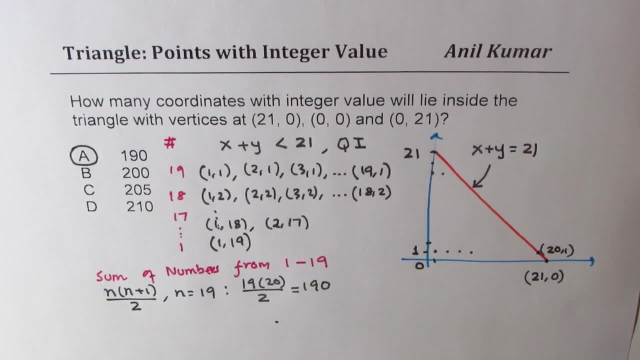 is one way of doing. you get the answer a the other way. for some of you is very interesting, those who have not learned this formula. how do we get this formula? so let me extend this. so, when we are adding the numbers, let's say one, two, three, so on. still, this is seventeen. 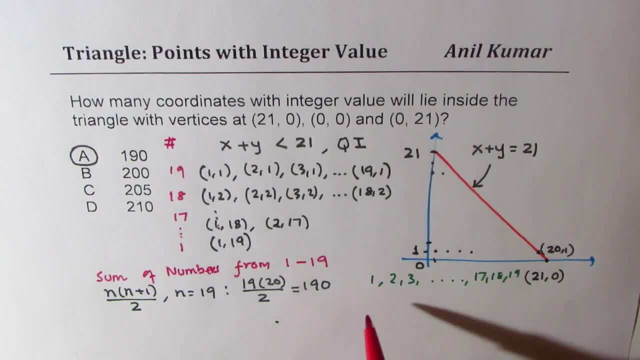 eight, nineteen, nineteen- we can actually group these right. so what is 1 plus 19? what is 2 plus 18 and what is 3 plus 17? we see all of them. when you add them, we get 20 correct. so so all of them: 19 plus one, 20 plus one: we get 20 of these correct. so this sum is equal to: 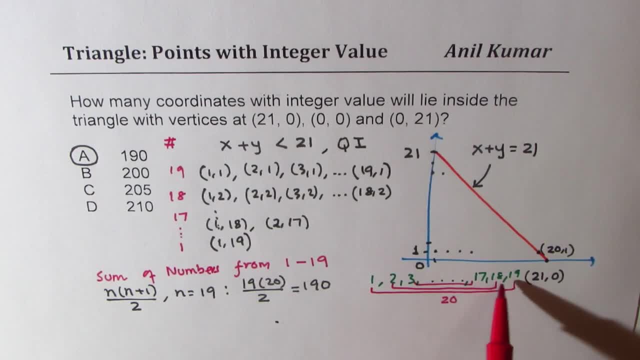 the sum is 20, and how many do we have in this combination? half of 19hem right? so? so show me, is 20 for set of 2, right? so since there are 19 numbers, half of 19 will be the number of sets. half of 19 means there will be one individual, 10. I mean lying just down.